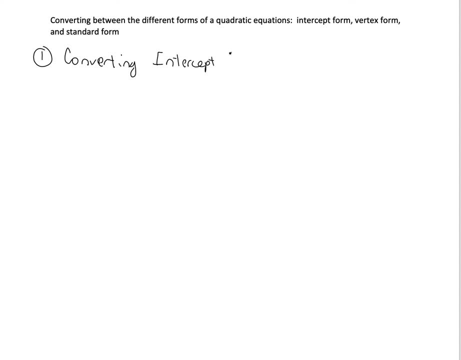 intercept form to standard form. Okay, so let's say you're given the equation, y is equal to 3x minus 4 times x minus 1.. This is an equation in intercept form And we want to make it into standard form. Remember, standard form is the equation in which you make the 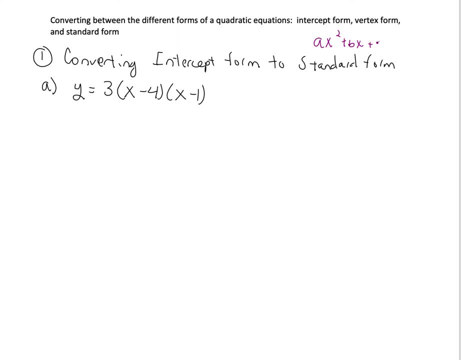 expression: a, x squared plus bx plus c equals y. And so to do this, we're just going to do our full method. So I'm going to start by taking the x minus 4 and times it by the x minus 1.. So I'm going to take x times x gives me x squared. Then I'm going to take: 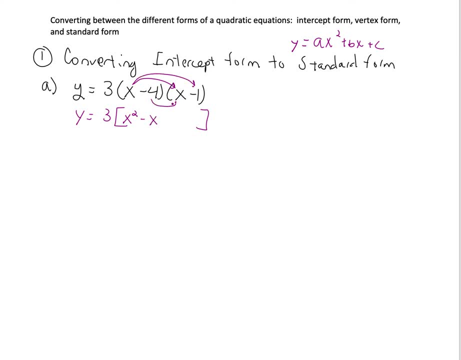 x times negative 1, give me a negative x Negative 4 times x is negative 4x And negative 4 times a negative 1 is plus 4.. Combining like terms, I end up with x squared minus 5x plus 4.. Then, last step, I'm going to do my distributive property and distribute. 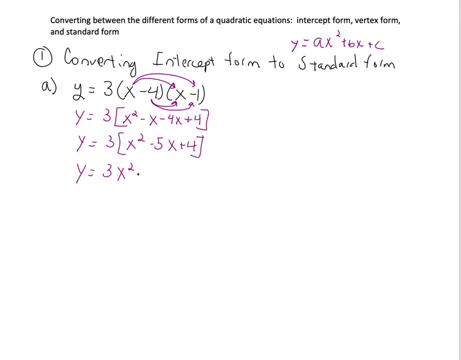 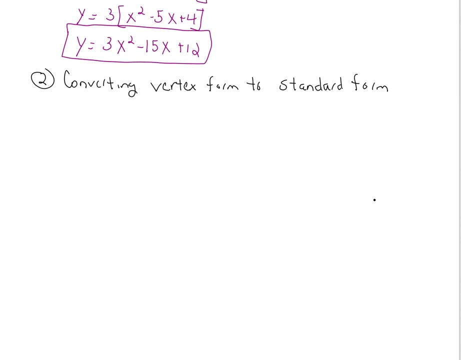 this a to every term. So it gives me a 3x squared minus a 15x plus a 12.. And I have now written my intercept form equation into standard form. Our second method is we're going to convert from vertex form to standard form. All right, 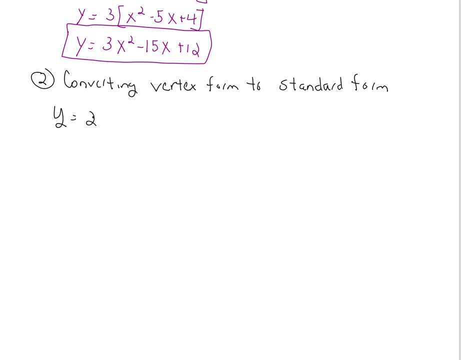 let's say we have the equation y e, Y equals negative 2x minus 1, squared plus 5.. So this is the equation in vertex form, vertex of 1, 1, 5. And we have an a of negative 2.. So to write this in standard form first: 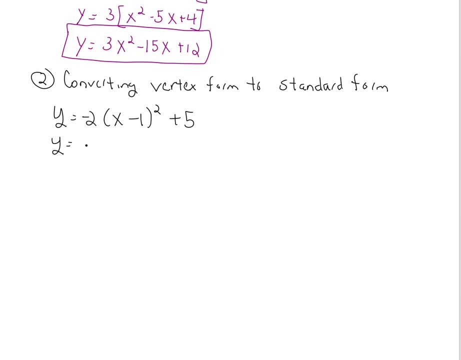 thing I realize is, when I have x minus 1 quantity squared, that means I have x minus 1 times x minus 1.. So I'm going to replace this x minus 1 squared with x minus 1 times x minus 1.. And I'm going to do pretty much what I just did in the last. 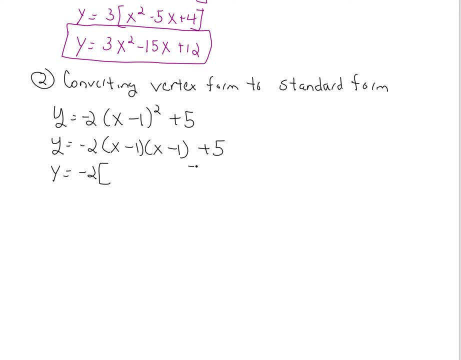 example, I'm going to start by doing my full method here, So let me change the color. So I'm going to take x times x. It gives me x squared, And then it gives me a negative x minus x plus 1.. 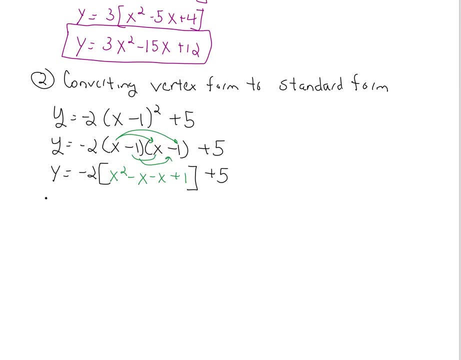 My next step. I'm going to combine my like terms so I have negative 2, and then my like terms end up being x squared minus 2x plus 1.. Our next step is the distributive property, and distributive is negative 2 to every term. 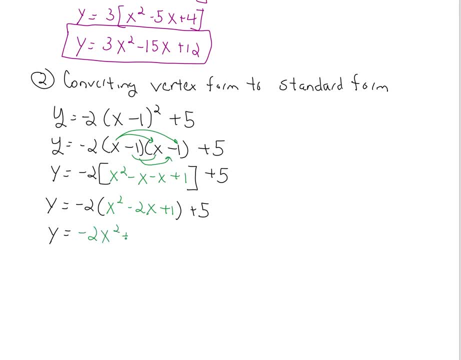 in the parentheses. So that's a negative 2x squared plus a 4x minus 2, keep that plus 5.. And my last step is: I'm going to combine any like terms. so I got negative 2x squared plus. 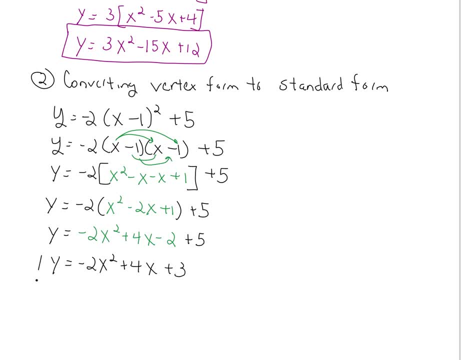 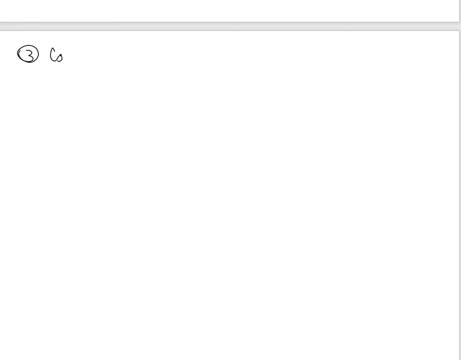 a 4x plus 3.. And I now have written this vertex form equation into standard form. Step 3, we're going to convert from standard form to intercept form. I'm going to do a couple examples in this form because, depending on how challenging, the problem is, it's going to be hard to find the right answer. So I'm going to do a couple examples in this form because, depending on how challenging the problem is, it's going to be hard to find the right answer. So I'm going to do a couple examples in this form because, depending on how challenging the problem is, it's going to be hard to find the right answer. 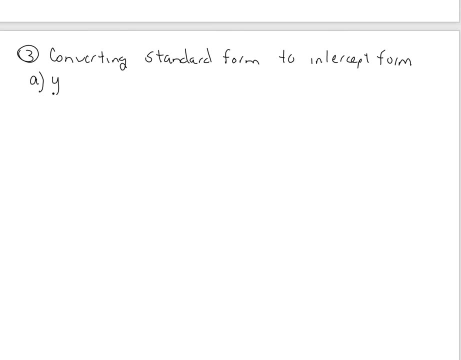 So let's milk of the first one. We got a 4x squared plus an 8x minus 12.. Now I'm converting from standard form to intercept form. intercept form has our two factors. Our key with this is we want to just factor the equation. so I'm going to learn. 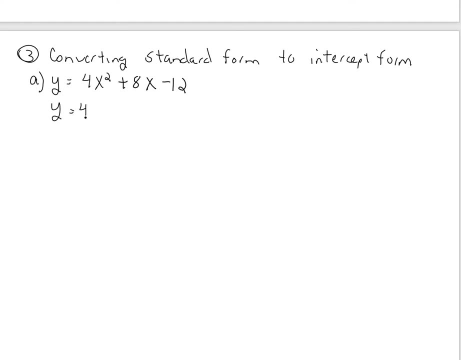 how I factor. The first thing I'm gonna look at is I have a gc2.. So I'm going to factor out that GCF of 4.. And that leaves me with X squared plus a 2X minus 3.. Now that I've factored out my GCF of 4, I'm going to look at these parentheses here and 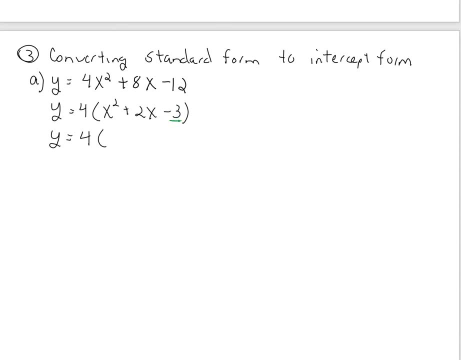 see if I can factor this down. So first thing I know is I need the factors of 3 that subtract to equal a positive 2.. So the only factors of 3 are 3 and 1.. And the only way I can get I can subtract these numbers to get a positive 2 is, I take 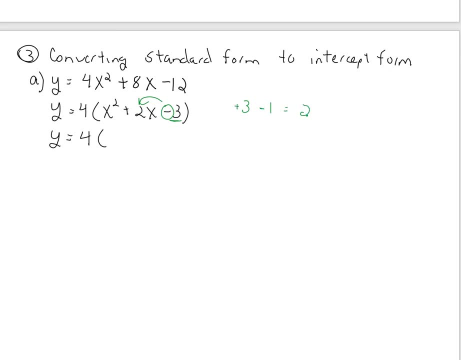 a positive 3 minus 1 and that's going to give me a positive 2.. So I'm going to replace this X squared, this 2X term, with a minus X plus a 3X, And then I'm going to factor this using my factoring by grouping. 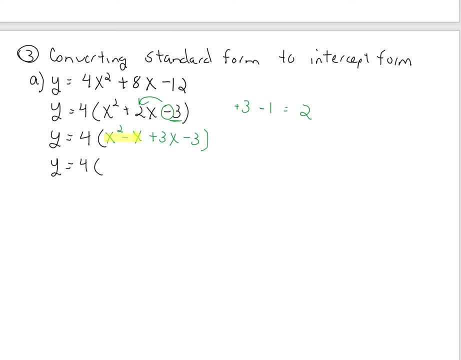 And my first set of parentheses here. if I look at these two terms, my GCF is X, so that leaves me with X minus 1 plus, because I always bring that sign down. And looking at my second two terms, my GCF is 3.. 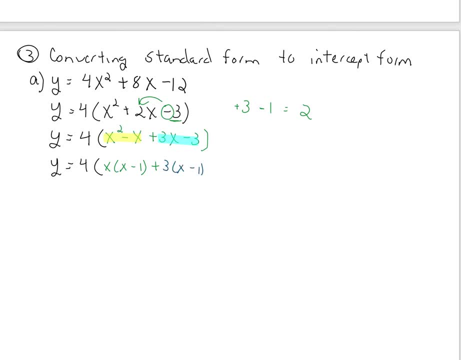 So that leaves me with X minus 1.. So I have my GCF now is X minus 1. And what's left over is X plus 3.. And now, So I've fully factored this and it happens to be in intercept form. 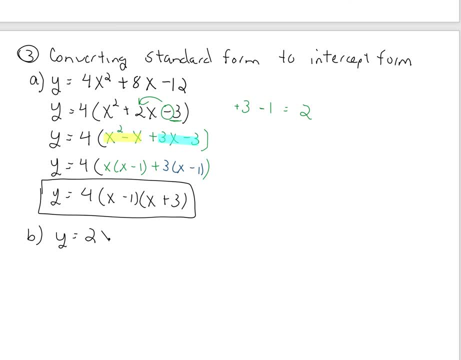 Second example: it's a little bit harder because I do not have a GCF, But I do have a number in front of my X squared term. So I have an A, Because I know in standard in our intercept form A has to be factored. 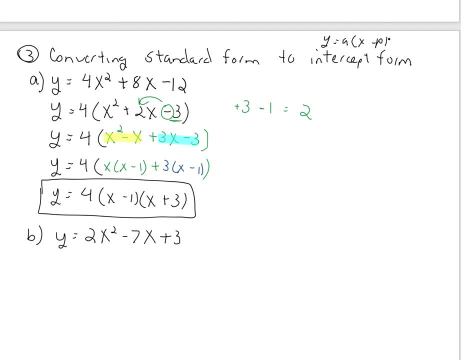 out. We cannot have a number in front of our X terms when it's in this form, Because our intercept form is A times X minus P, times X minus Q, And there's no number in front of those X's. So this is what makes this one a little bit more challenging. 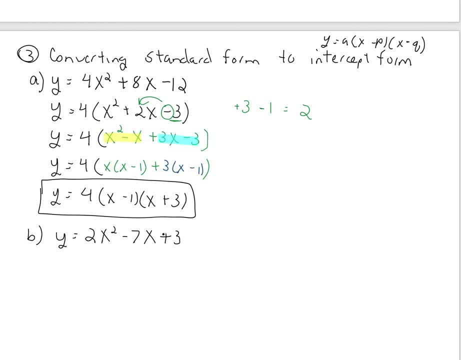 I'm going to start the same way. I'm going to try factoring it first. Looking at this, I know I multiply my outside numbers together And that's 6.. So I list all the factors of 6.. That's 1 times 6 and 2 times 3.. 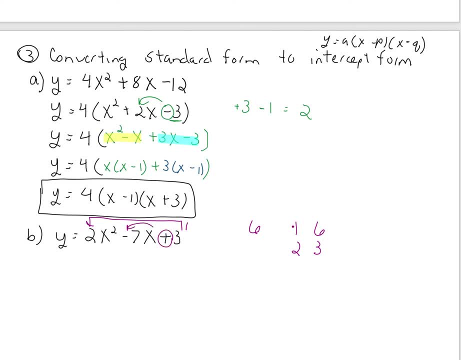 And I want to know the ones that add to equal a negative 7.. Well, that would be a negative 7.. Negative 1 plus a negative 6,, which will give me a negative 7.. So I'm going to go here and replace that middle term with my two factors of a negative 6X. 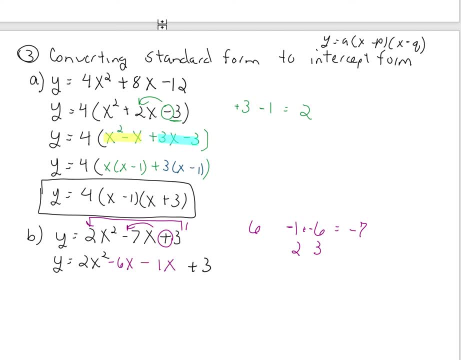 minus 1X. And then I'm going to look at that. I'm going to look at my first two terms and factor out my GCF there, which is a 2X. Taking out a 2X, that leaves me with an X minus 3.. 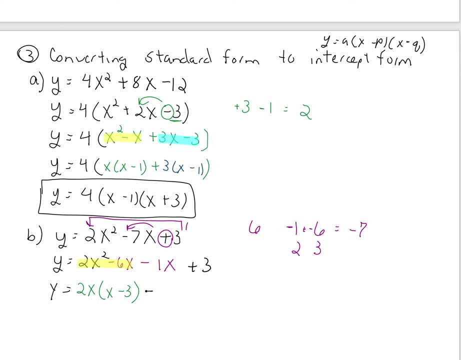 Bringing down my negative sign. that sign always comes straight down, So I'm going to have to factor out a negative. Then I'm going to look at my next two terms. factor out that GCF, where there's nothing in common. So I'm going to factor out a 1,, a negative 1, which gives me an X minus 3.. 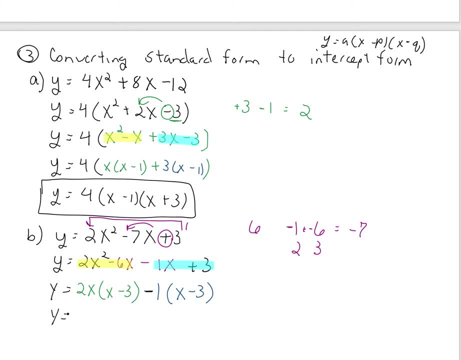 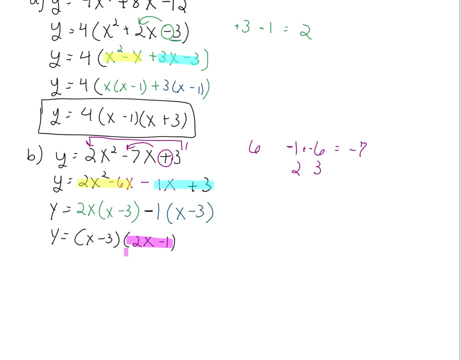 Putting these together, I get the X minus 3 is a common factor and that leaves me with a 2X minus 1.. If you look this, 2X minus 1 is a problem because we cannot have a number in front of. 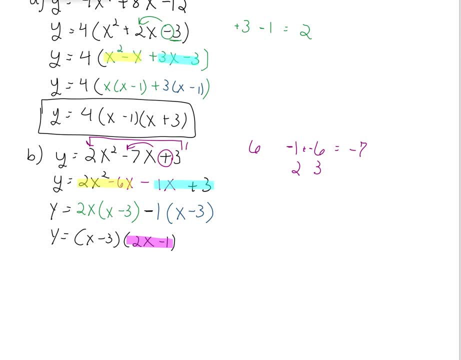 that X, Easily solved. All we're going to do is we rewrite this parentheses and I'm going to factor out whatever that A term is. I'm going to take 2 out of only this parentheses. So if I take a 2 out, 2X divided by 2 is X. 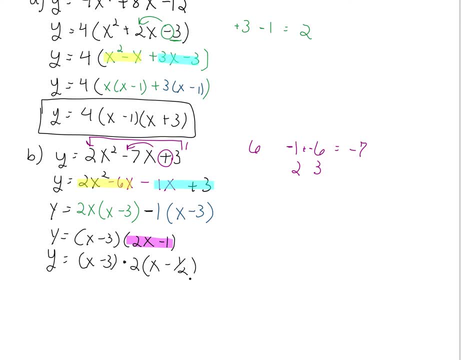 If I divide 1 by 2, that gives me a 1 half. Then I'm just going to rewrite this in my form. That constant goes in the front And then my two factors. So this intercept form of this equation is: Y equals 2 times X minus 3 times X minus 1.. 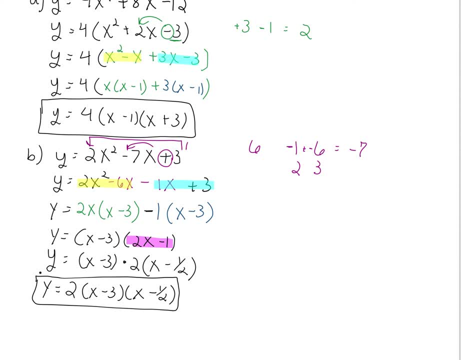 So I'm going to take 2 out of only this parentheses, It's going to be 4 times X minus 1 half. So I'm going to write it: 2 times X minus 1 half. This is going to be a normal sum. 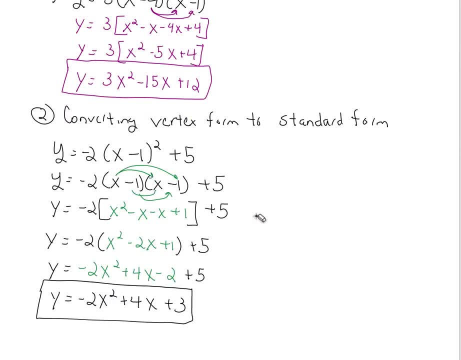 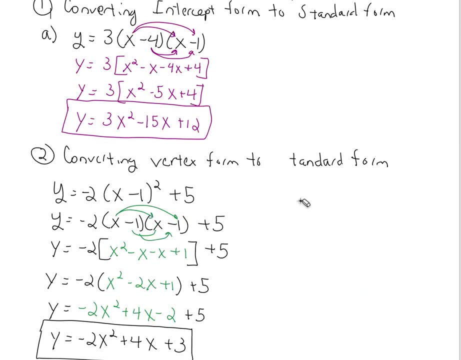 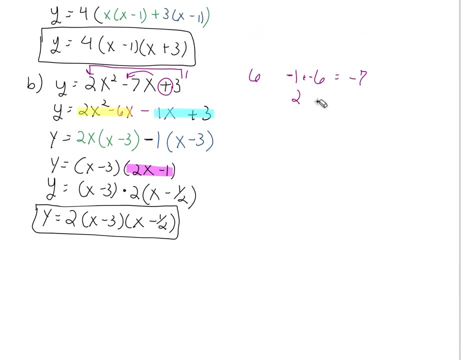 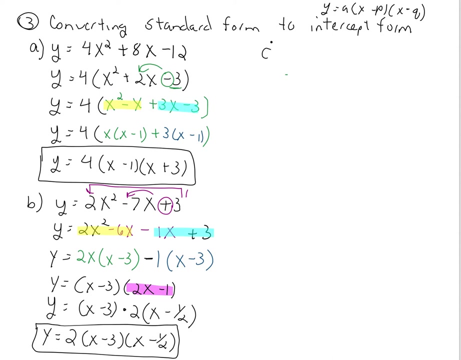 It's going to be negative 2 times X minus 1 half. Let's do one more. That is so annoying. I don't know why it's giving me such a problem. Let's see. Let's see, We have our Sx. 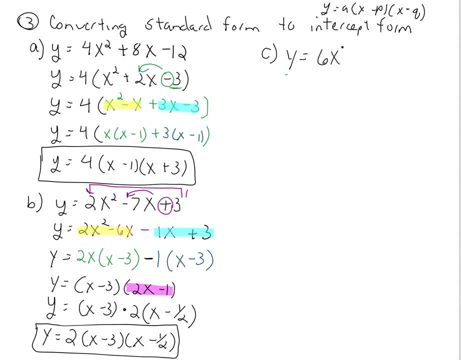 In this example we're given y is equal to 6x squared plus 13x plus 5.. I'm going to write this in intercept form, So I'm going to start by factoring it. I got my factors of 30 that add to equal 13.. 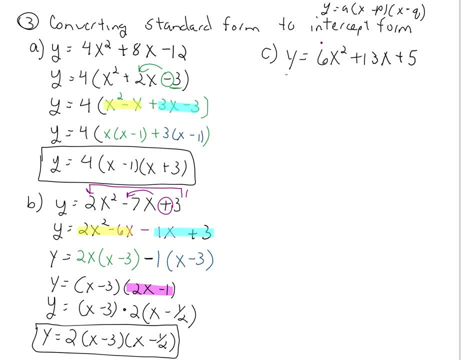 So let's see: Multiply these together. So 5 times 6 is factors of 30. That's 1 and 30, 2 and 15.. Oh there we go: 3 and 10.. And those are the ones that add to equal 13, because 3 plus 10 gives me 13.. 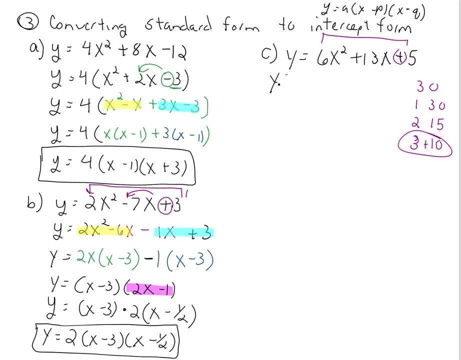 So when I rewrite this I'm going to do: y is equal to 6x squared, Replacing the 13x with a 3x plus a 10x, Taking the GCF of the first two terms and I can factor that out. 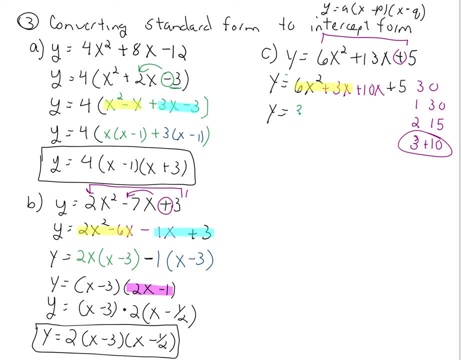 And I see I can factor out a 3x and that leaves me with a 2x plus 1.. Then I want to look for my GCF of these two terms, Again, the plus sign has to come down. 5 is in common. 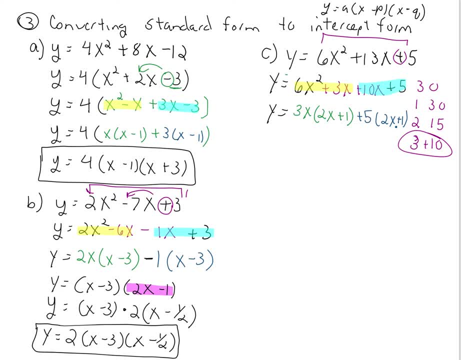 So it leaves over 2x plus 1.. Yes, what's in parentheses is the same, So I can rewrite this as y is equal to 3x plus 5 times 2x plus 1.. But again I have problems. 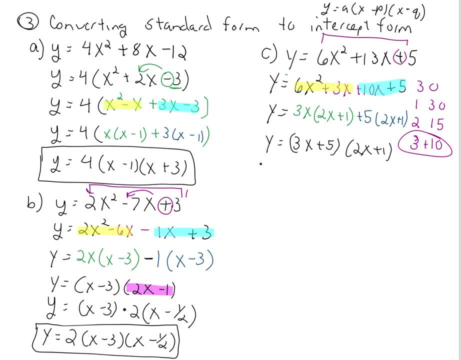 I have a number in front of my x and a number in front of my x here, So I have to factor out a 3 from the first parentheses, which gives me x plus 5x, 5 over 3.. And then I have to factor out a 2 from my second parentheses. 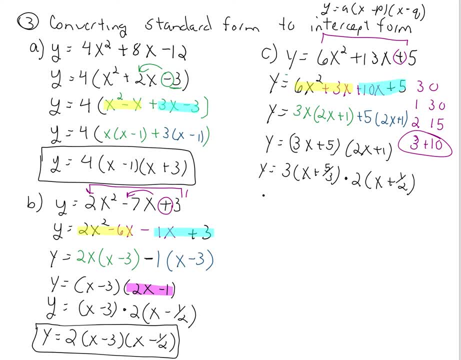 which gives me x plus 1 half. I have a 2 and a 3 factored out, so it multiplies together. It equals 6x plus 5 thirds times x plus 1 half. This is the most complex way that you're going to have to convert. 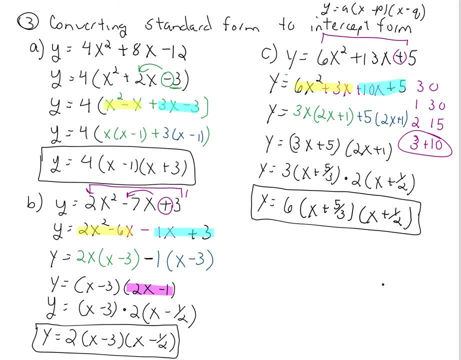 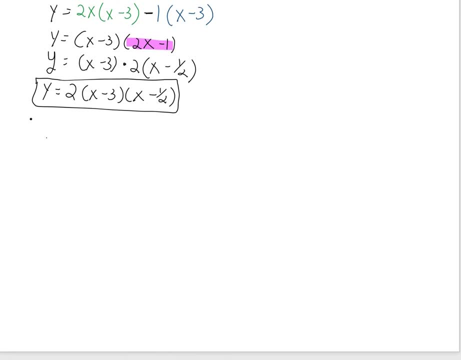 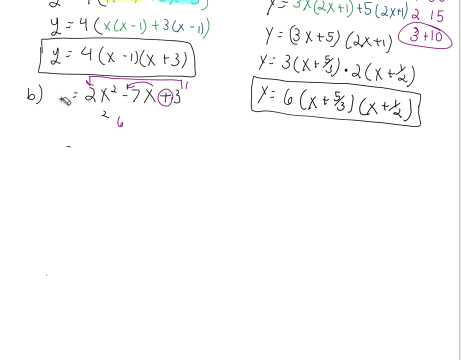 from standard form into intercept form. Our last type of conversion? All right. so our last type of conversion is when we're going to convert from standard form to intercept form. All right, So our last type of conversion is when we're going to convert from standard form to intercept form. 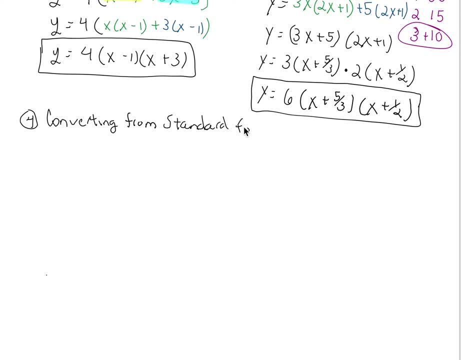 to vertex form, So that's y equals ax squared plus bx plus c. to vertex form, which is y equals a, parentheses, x minus h, squared plus k. So the final answer needs to look in this form: The method we're going to use to do this is: 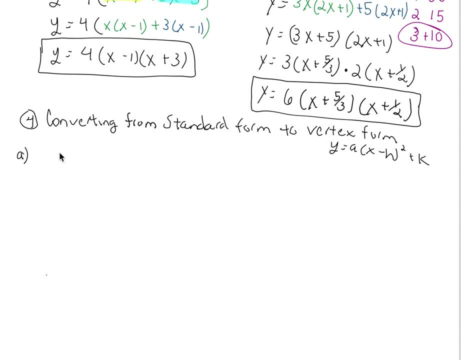 called complete the square. And again I'm going to do a couple examples, because this one can be a little bit more complex based on the problem. So we'll start with the most simple type. Alright, so we're given y is equal to x squared plus 4x minus 1. 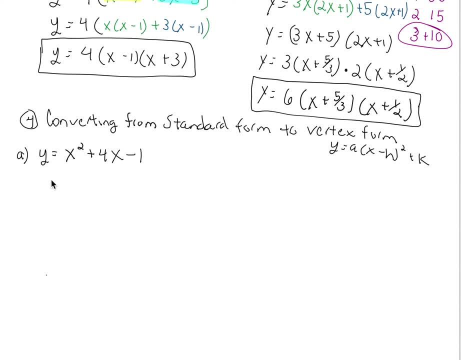 and we want to complete the square on this. Step one is you're going to group your x squared terms, your x terms together, Any terms that has x put in parentheses. That's your step one. Step two: if there's a number besides one in front of the x squared, you factor it out. 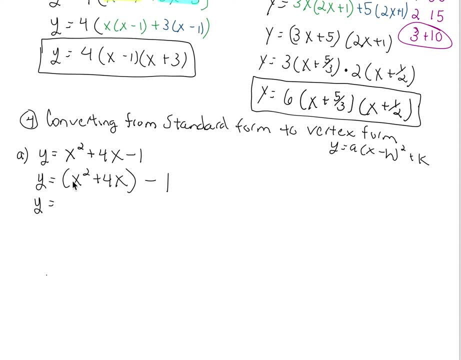 In this case I don't have any number in front of the x squared, so I can skip that step and move on to step three, which I say I call it setting up your blanks. So I got x squared plus 4x and I want to add some number to this. I don't know what that number is yet. 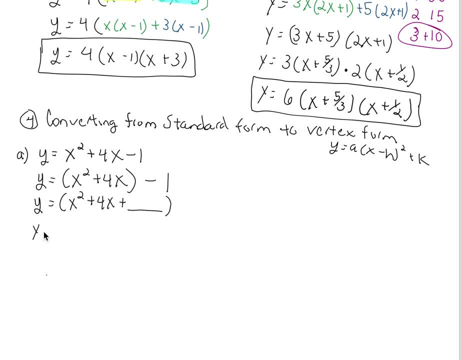 so that when I factor this it becomes something squared. So something times itself. So this factors into a perfect square. But if I set up this equation and I add some number to this inside the parentheses, I therefore have to subtract some number from the equation. 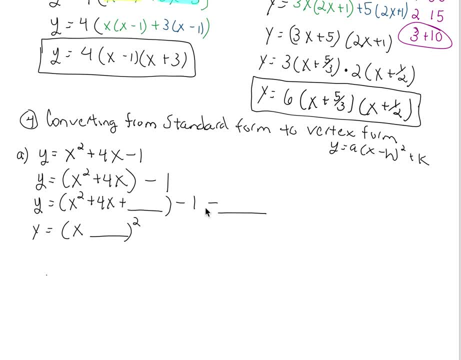 Because if I add something and subtract something, I have not changed my function at all, So I have to keep it balanced. Anything I add, I have to subtract, And so now this is the blanks. These two steps here are the setting up, the blanks. 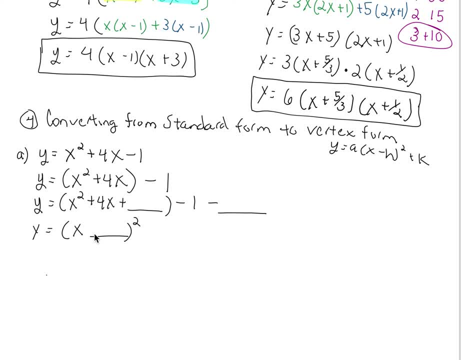 And we have to figure out what goes into the blanks. This bottom blank is what I usually fill in first, Because I look at my b term. Whatever this sign is, that sign comes down, Then I take that 4 and I divide it by 2.. So, whatever the b is, 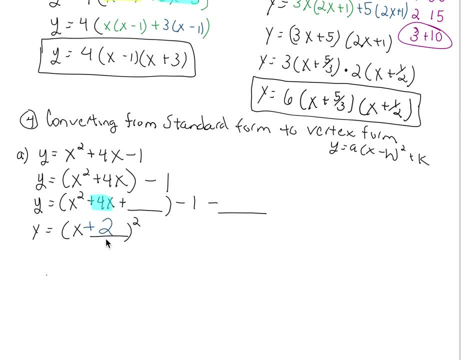 divide it by 2 and that gives you this bottom blank. So 4 divided by 2 is 2.. Then I take 2 and I square it and it goes into this blank. This is why this is always positive, Because even this is negative 2.. 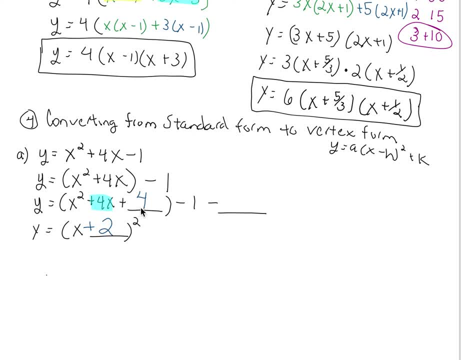 Negative 2 times negative. 2 is positive, So it's always going to be a positive term here. So now I've added 4 to the inside of the parentheses. So since I've added 4 to the inside, I need to subtract 4 from the outside, And then all that's left to do is combine my 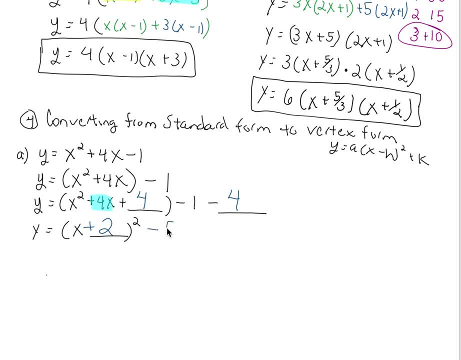 like terms. Negative 1 minus 4 is actually a negative 5 on the outside. And you are done. You have used complete the square to transform the standard form into vertex form. Our next equation is 2x squared plus 4x plus 3.. 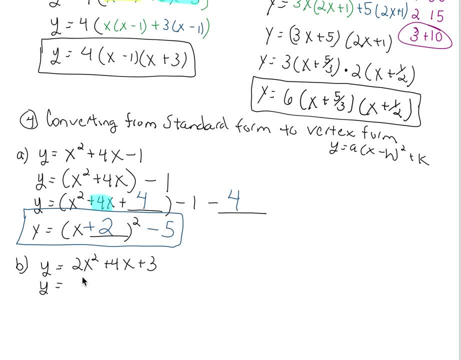 Start the same way. We want to use complete the square to write this in vertex form. So I'm going to group all my x terms together, But this time I have a number in front of my x squared, So I must factor that number out. 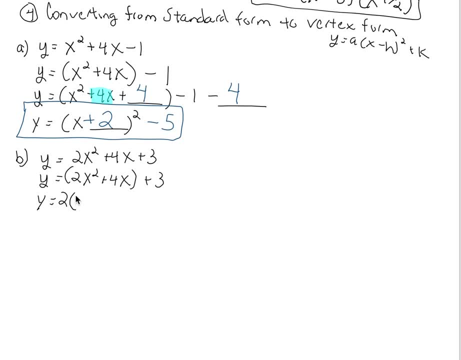 So I'm going to take the 2 out, And that leaves us with x squared plus 2x. Now that I don't have a number in front of this x squared inside the parentheses, I'm ready to set up my blanks, Copying down everything down. 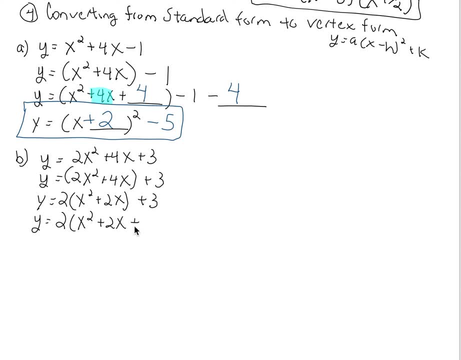 So I've got x squared plus 2x. I'm going to add something And then, whatever I add, I need to subtract from my equation And I'm going to do something to make it a perfect square. So I'm going to set this parentheses so that I have a perfect square. 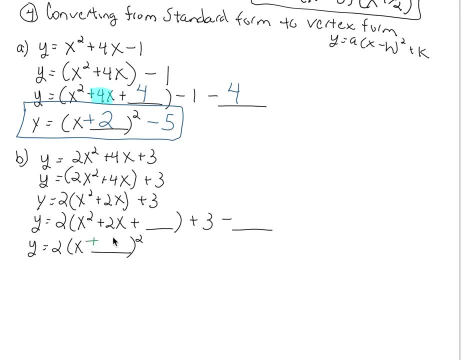 So I have a plus sign. So my plus sign needs to come down: 2 divided by 2 is 1.. 1 squared is 1.. Now here's where this one's a little bit different. I did not add 1 to this problem. 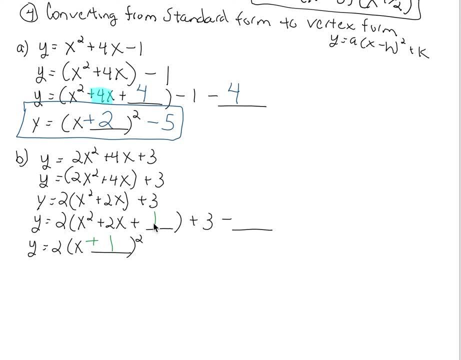 Because, remember, I have this 2 on the outside, So that means I have to distribute this 2 to everything, in parentheses. So I've actually added 1 times 2. Which is 2 to the problem. So I need to subtract 2x. 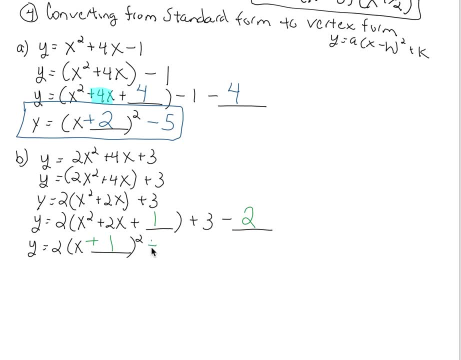 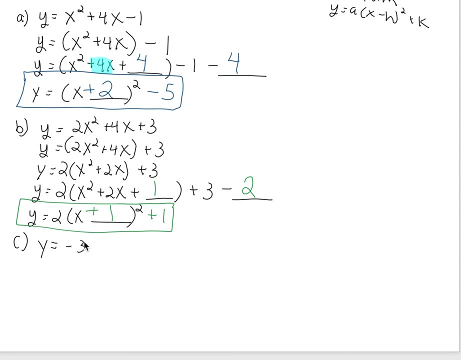 2.. Then, combining my like terms, I get a plus 1.. So this would be the equation in vertex form. Alright, the last one. The most complex way that you might see this Is: let's say, I have a negative 3x squared. 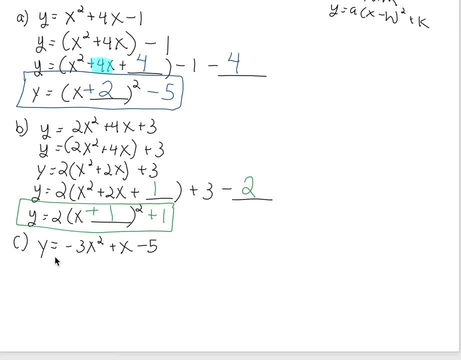 plus x minus 5.. And you're asked to write this in vertex form, So the steps are the same. I'm going to start by grouping my x squared terms, My x squared term and my x squared term. So I'm going to start by grouping my x squared term and my x squared term. 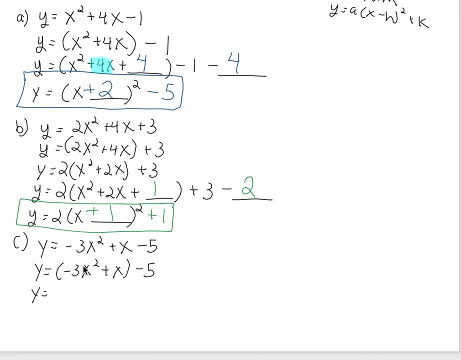 Then I'm going to factor out whatever's in front of the x squared, So it's a negative 3.. Now what makes this challenging is this: negative 3 does not divide equally into a positive 1. That's okay, You can use fractions. Fractions are our friends. We love them. 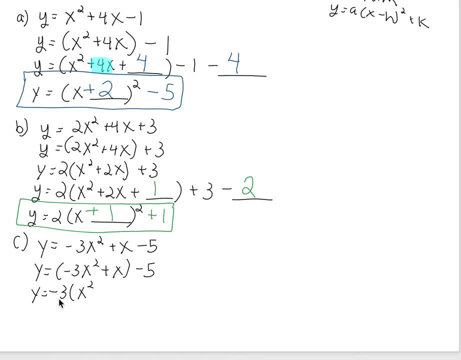 So if I take this positive 1x and divide it by a negative 3, I get a negative 1 third x. So that's what's going to be in the end. So I'm going to write this in my parentheses here: 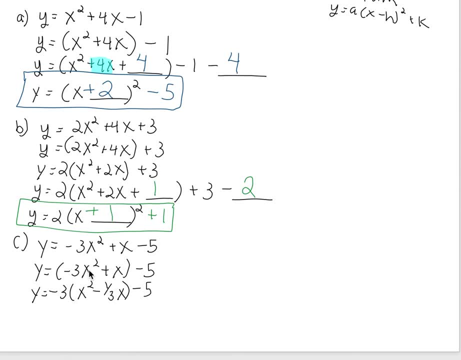 And you can check that: Distribute property. If I distribute this, I get negative 3x squared, Negative 3 times a negative. 1 third x gives me a positive x. So it's still balanced. The equation hasn't changed any. 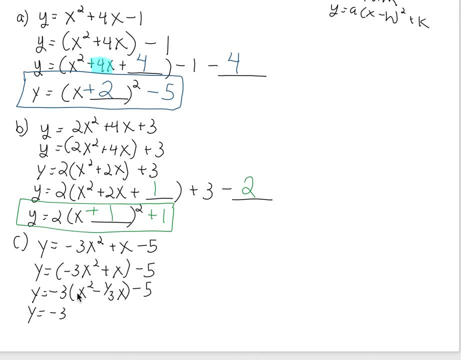 Now that I have an x squared term with only a 1 in front of it, I can set up my blanks. I'm going to add something inside- That means I need to subtract something on the outside, And I'm going to make this bottom so it's something completely squared. 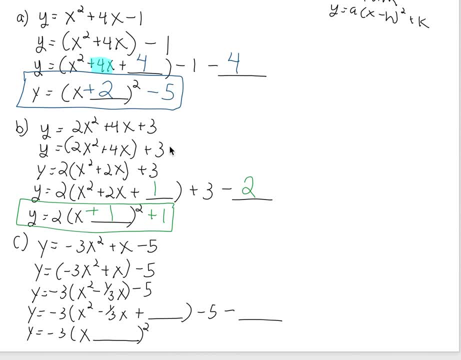 So our procedure again is we take this b term, negative 1 third, and divide that by 2.. So that gives me a negative 1 sixth. 1 third divided by 2 is 1 sixth. Now I take this negative 1 sixth and I square it. 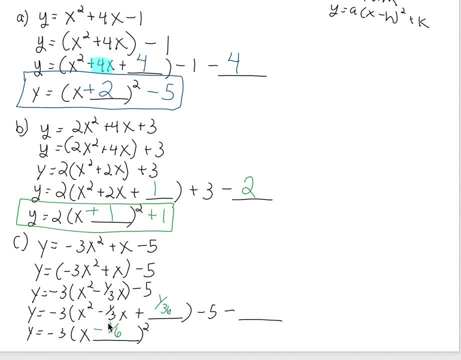 That gives me a positive 1 over 36, because I squared the top number and squared the bottom number. Then a positive 1 over 36 times a negative 3 gives us a negative 1 twelfth Now, since I am actually subtracting 1 twelfth from this problem. 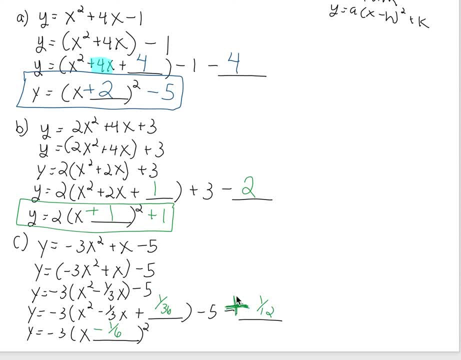 I now have to change this to a plus sign. Minus a negative equals a plus sign, Because this is actually subtracting, not plus, like I had been doing in these other problems. So now let me give myself a little room. over here We have: y is equal to negative, 3x minus 1, sixth squared. 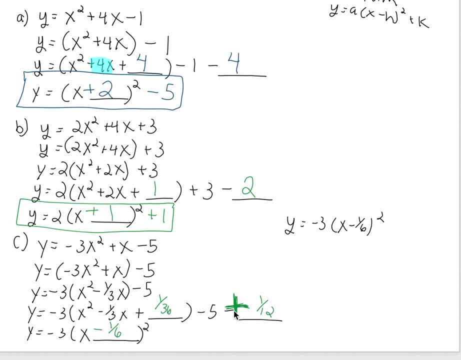 And I need to combine these two terms. So to combine these, I need a common denominator So I can rewrite negative 5 as 60 over 12 plus a 1 twelfth, And so that's going to give me negative 3 parentheses, x minus 1 sixth, squared minus 59 twelfths. 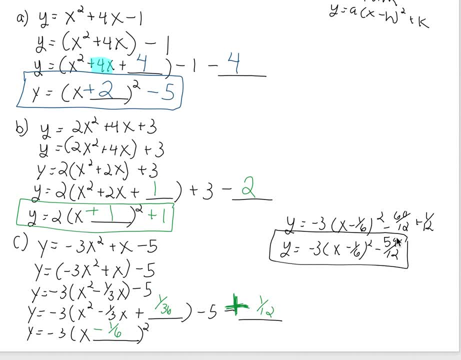 And now I've rewritten this standard form equation into vertex form. I hope this helps you when you're converting in between the three different forms of the quadratic equation.